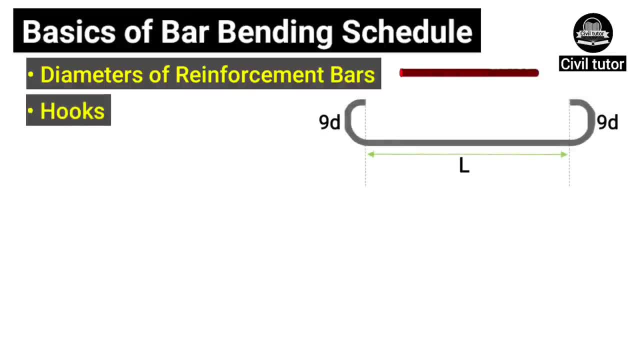 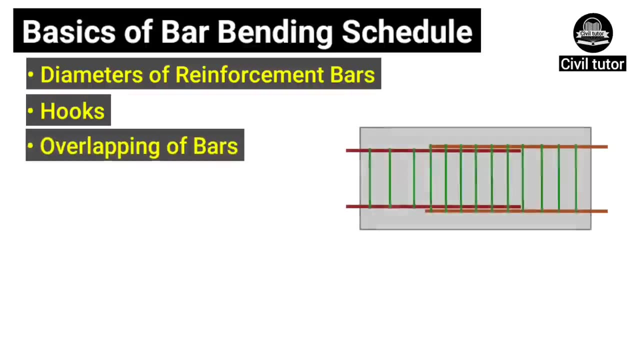 The next topic will be about hooks, in which we will discuss the reasons of providing hooks in structural members, the function of hooks in city ropes and how to calculate the hook length and cutting length of bend. I am going to discuss about the provision of overlapping of reinforcement bars in structural 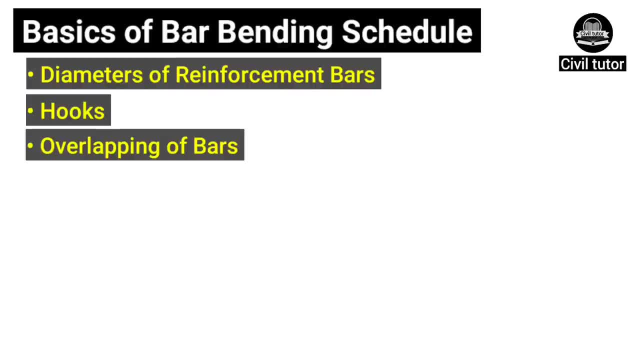 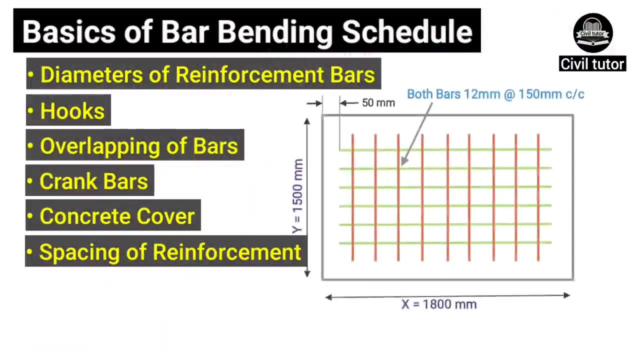 members, This lecture will also include the provision of crank bars and how to calculate the cutting length of cranked bars. I am also going to discuss about concrete cover Spacing of reinforcement bars, how to calculate the number of bars, number of city ropes and. 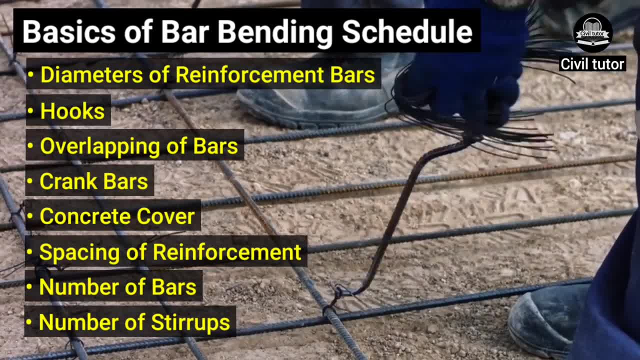 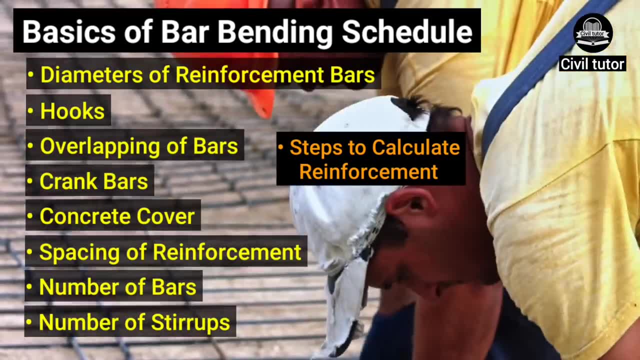 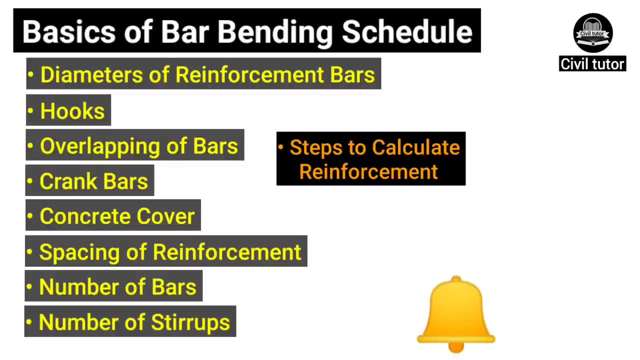 at the end of this lecture, the most important discussion will be about the basic steps used to calculate the reinforcement details of a structural member. So before starting this lecture, if you haven't subscribed my channel, please subscribe it, and don't forget to press the bell icon so that you don't miss any updates in future. 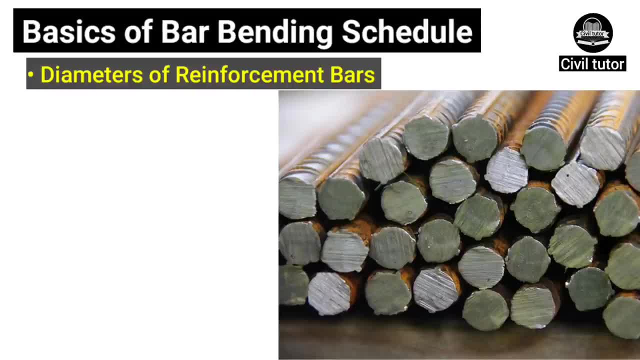 The first topic is about diameters. Reinforcement bars are available in various sizes, in which we have 6mm, 8mm, 10mm, 12mm, 16mm, 20mm, 25mm, 28mm, 32mm and 40mm dia bars. 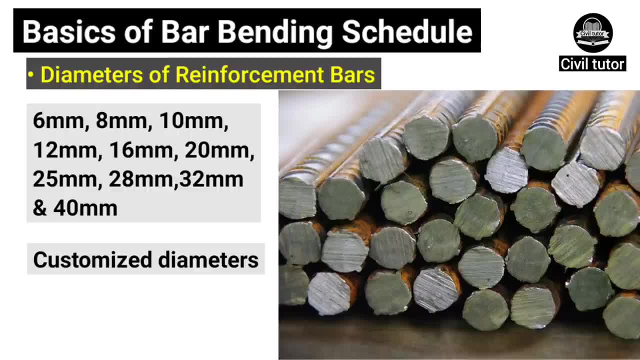 In addition to that, we can have customized diameters which can be ordered directly from the industry as per our need. The standard length of a diameter is about 1.5mm. The diameter of a diameter is about 1.5mm. 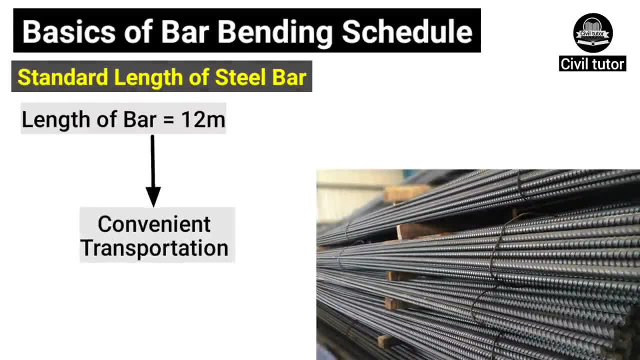 The diameter of a diameter is about 1.5mm. The diameter of a diameter is about 1.5mm. Moreover, the diameter of a�m bar is usually kept as 12m for convenient transportation, or this can also be customized as per the bar bending schedule, which is usually done. 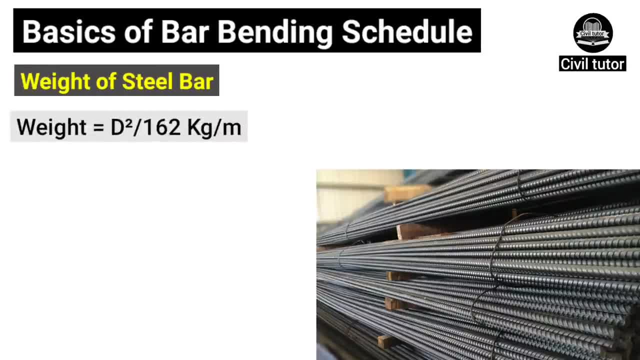 in megaprojects. The weight of a steel bar is calculated by using the formula d2 upon 162 kg net per meter, in which d is the dia bar. For example, if we have a bar of size 8mm, its weight in kg per meter will be equal to. 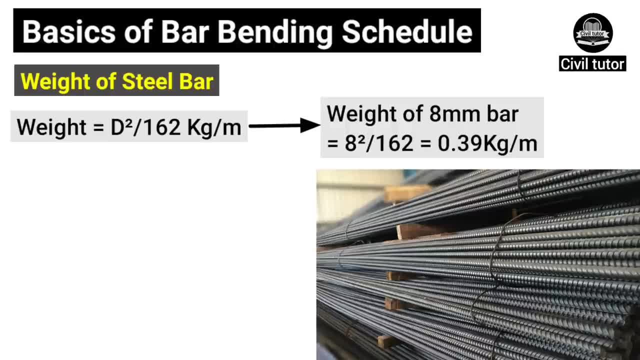 82 upon 10k 162,, which will be equal to 0.39 kg per metre. Weight per bar will be equal to d square upon 162 into 12,, while 12 is the standard length of steel bar. For example, weight of 8mm steel bar will be equal to 8 square upon 162 into 12, which. 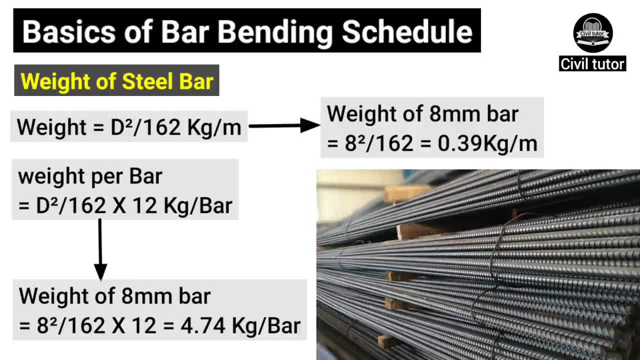 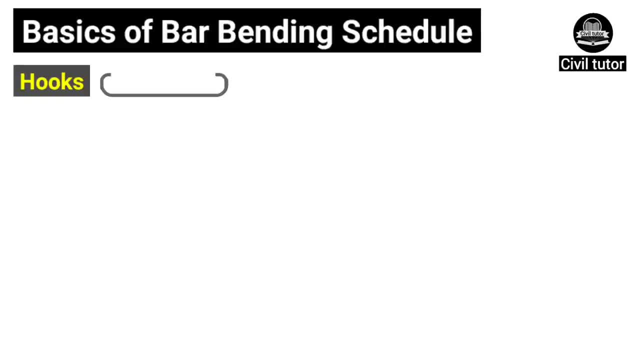 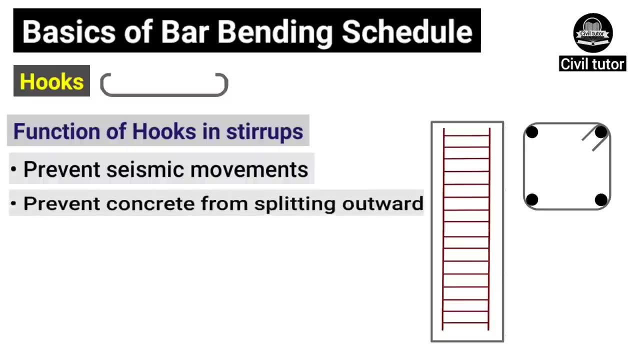 will be equal to 4.74 kg per bar. The next topic is about hooks. Hooks are provided in structural members as per the requirement. The function of hooks in city ropes is to prevent the seismic movements and to prevent the concrete from splitting outward. 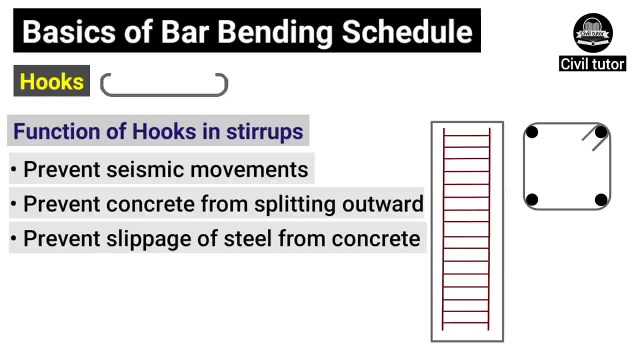 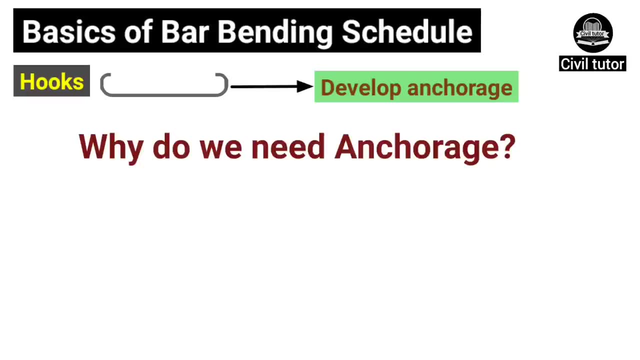 These also prevent the slippage of steel from the concrete. They keep the longitudinal bars in position and hold the steel tightly. The main function of a hook is to develop anchorage. Now the question arises: why is there a requirement for anchorage? 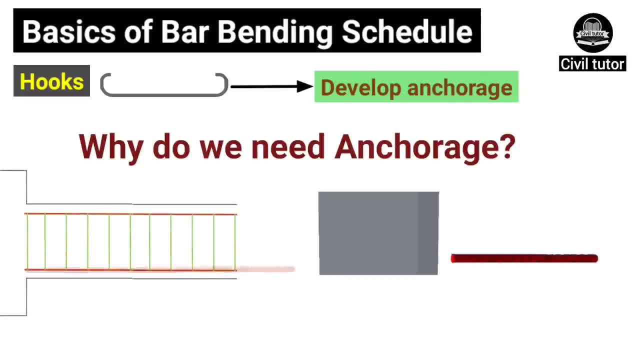 The tension reinforcement should not be slivered from its position, otherwise the purpose of providing the reinforcement will not be served. So to develop the sufficient bond strength between steel and concrete, development length requirements must be satisfied. Now there may be cases where there is unavailability of required length to meet the requirements. 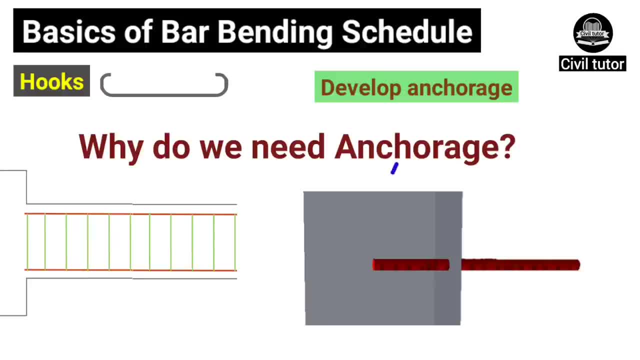 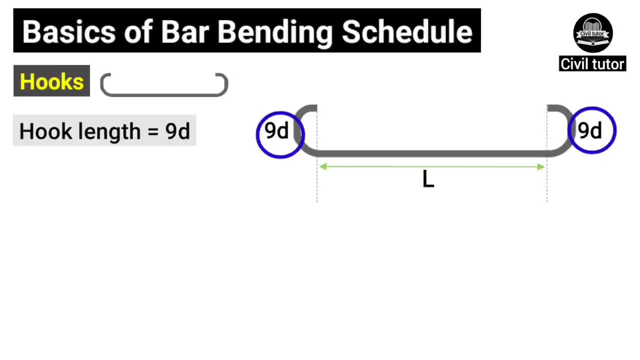 of development length. In those cases, anchorages may be provided in the form of hooks. The length of hook is calculated by using the formula 9 times D, while D is the diameter of bar. For example, if we have a bar of length L and the bar is provided with two number of 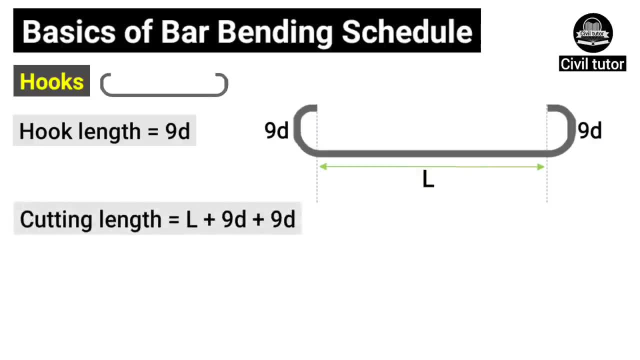 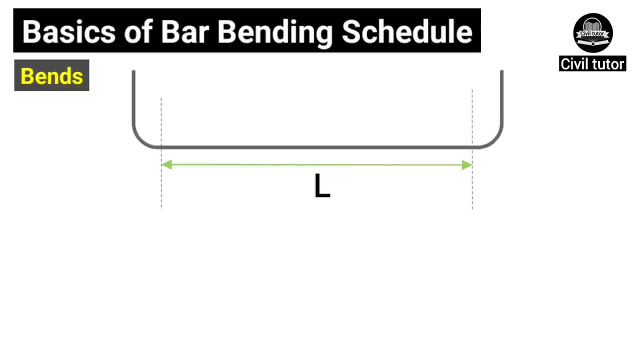 hooks on either ends. Cutting length of this bar will be equal to length of bar, that is, L plus hook length on either ends, which will be 90 plus 90.. The next topic is about bends. As you can clearly visualize from this picture, this steel bar is bent up on either ends. 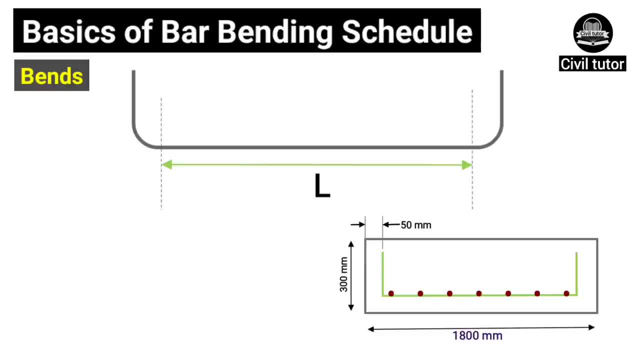 And these shapes are usually used in footings. The length of this bend is taken from 10D to 16D, in which D is the diameter of bar. The cutting length of this type of bar will be equal to straight length, L plus two number. 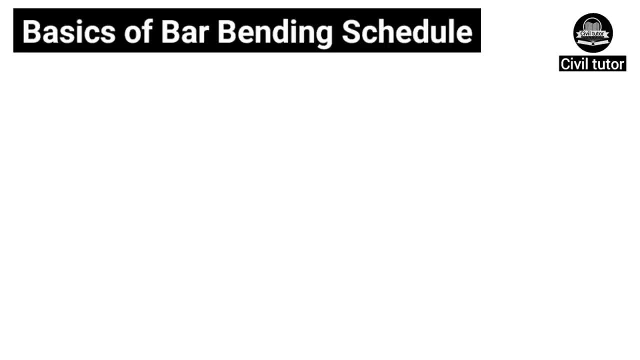 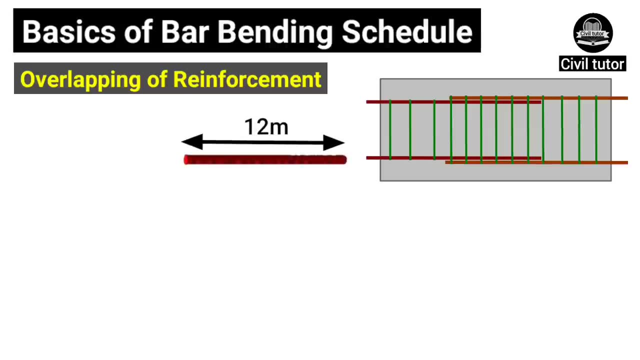 of bends say 12D plus 12D. Let's try this, See. The next topic is about overlapping. As we know, the standard length of a reinforcement bar is 12 meter, In case we need to increase the span of a. 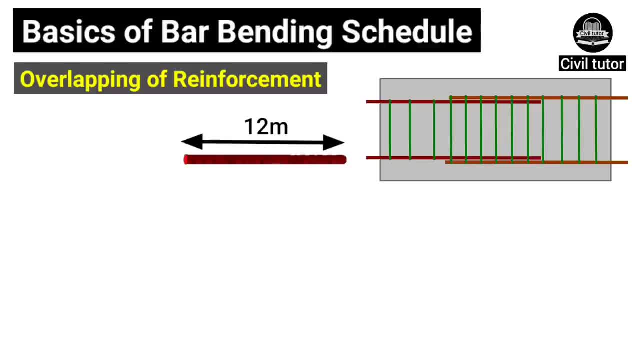 structural member, like beam or column, beyond the standard length of reinforcement, which means we also need to increase the length of steel bars by adding more reinforcement bars. If we add the straight bars directly from end to end, then there may be chances of slippage of steel, which is prevented by 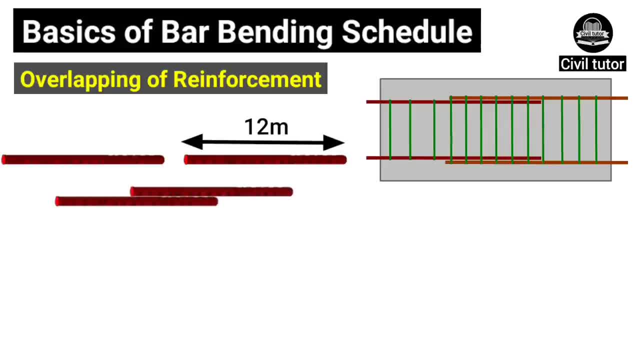 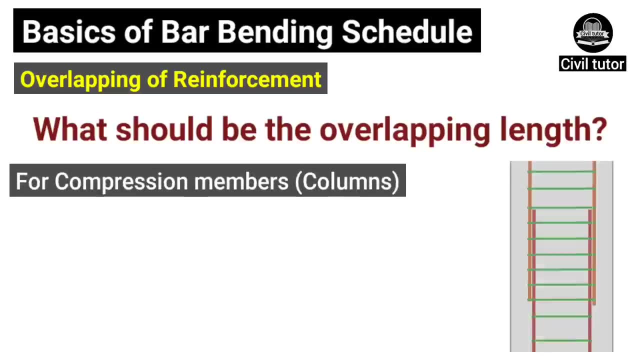 overlapping the bars. The purpose of overlapping is to retain the continuation of the steel bars to securely transmit the load from one steel bar to another bar. Now the question arises: how much should the overlapping length be taken? For compression members, that is, columns, the lap length should be taken as 40D, while D is the diameter of bar. 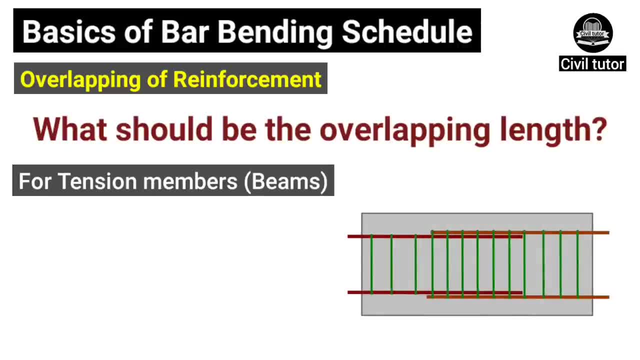 For compression members, that is, columns, the lap length should be taken as 40D, while D is the diameter of bar, And for tension members, that is, beams, the overlapping length should be taken as 50D. but from the practical point of view we can take 50D for both columns and 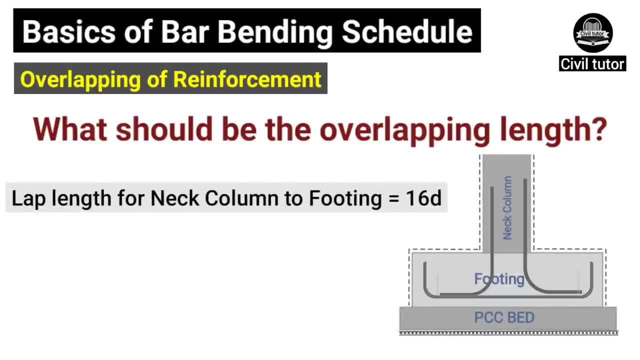 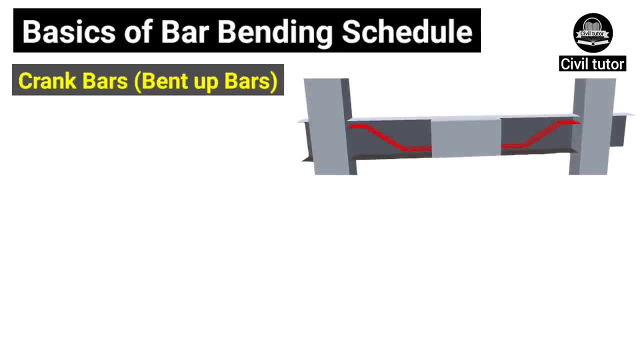 beams. If we need to overlap the reinforcement from neck column to footing, the lap length should be taken as 16D. This length is also known as development length. The next topic is about crank bars, Or bent up bars. Crank bars are those bars which can resist a negative bending. 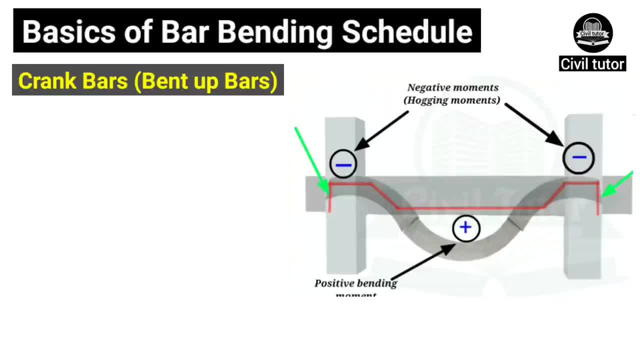 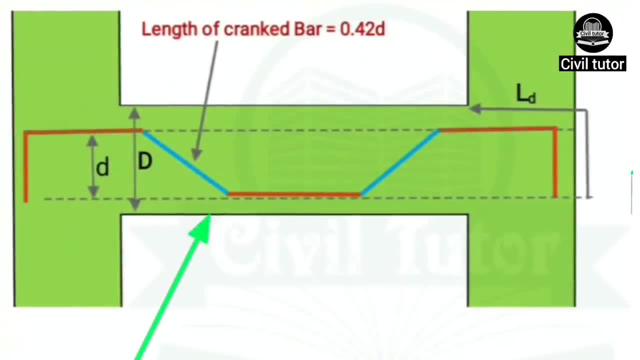 moment, or simply hogging moment. Bent up bars are provided in slabs as well as in beams, since these members are subjected to tensile stresses. For illustration, I have created a detailed section for a bent up bar. as you can clearly visualize from this picture, This inclined length is known as crank length, and 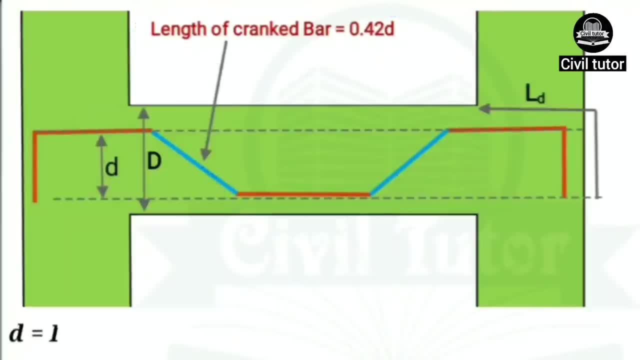 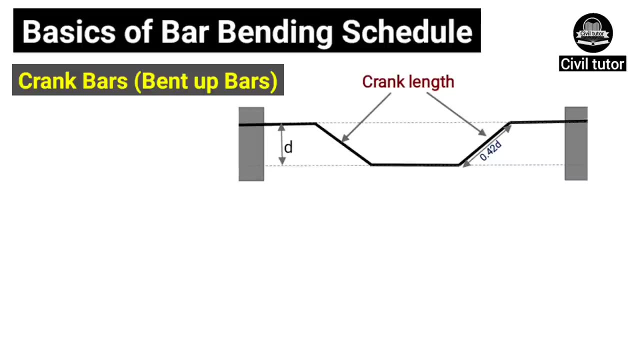 is equal to 0.42D. This D is equal to slab or beam thickness minus top and bottom cover. The cutting length of cranked bar is equal to span L plus 2 times crank length, that is 0.42D plus 0.42D. The next topic is about concrete. 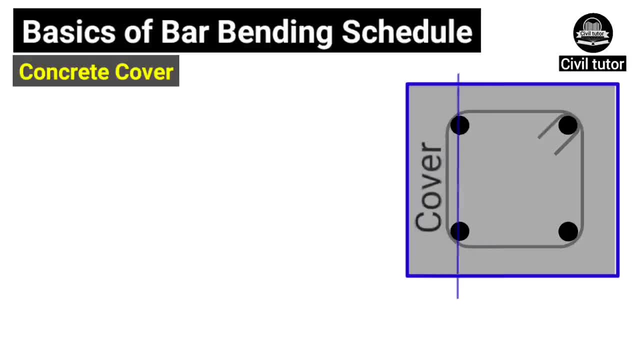 cover. Concrete cover is the space between reinforcement and shuttering, or it is the minimum distance between the surface of embedded reinforcement and the outer surface of concrete. The purpose of providing the concrete cover is to prevent the reinforcement bars from getting corroded by environmental exposure. Concrete cover provides thermal insulation to the steel. hence 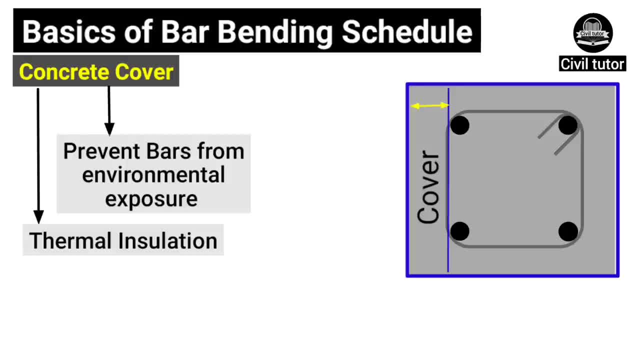 protects the reinforcement bars from fire. The minimum cover for footings is taken as 50 mm. For columns and beams, the minimum cover is taken from 25 mm to 50 mm and for slabs, the minimum cover is taken as 25 mm. For illustration, I have shown the cross section of a beam which 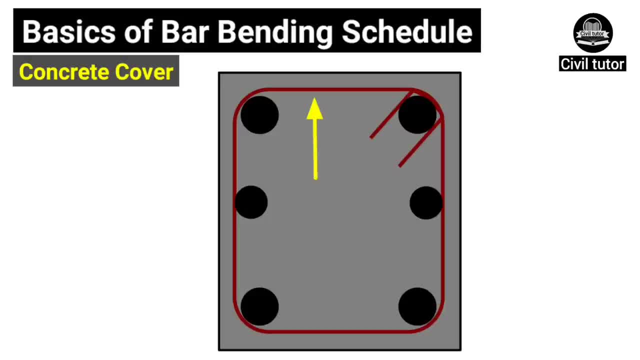 is of rectangular shape. This red color rectangle is the stirrup and the black colored circles are the main bars. The space between stirrup and outer surface of the beam is known as concrete cover, and the outer surface of the beam is the exposed concrete surface For providing the clear cover covering 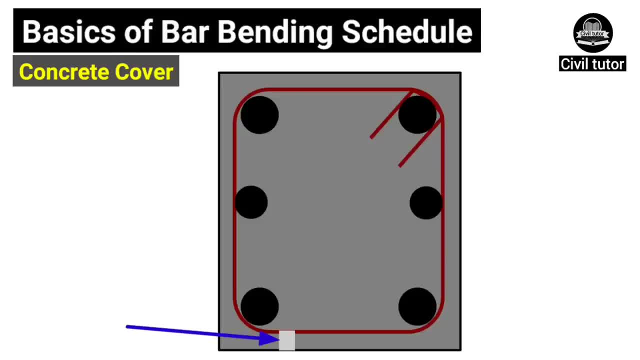 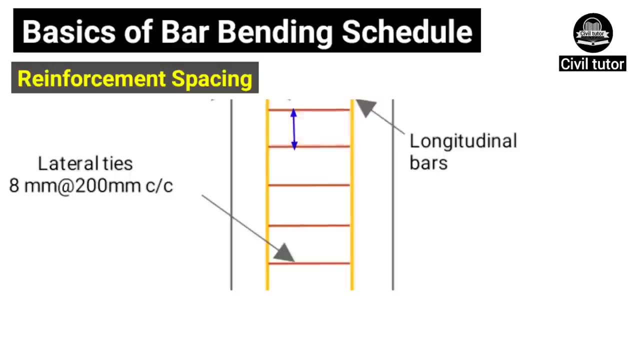 blocks are used to create a space between the reinforcement and the shuttering surface. These blocks are available in different sizes as per the need. The next topic is about reinforcement spacing. Spacing is the distance between two reinforcement bars. The spacing is provided to have a properly anchored reinforcement. That's why it's mandatory to cover the reinforcement physical of the rusher sociales. Spacing is provided to have a properly anchored reinforcement As per the needs required For this space, which is placed between the space of the reinforcement. the spacing should not have locationrs. 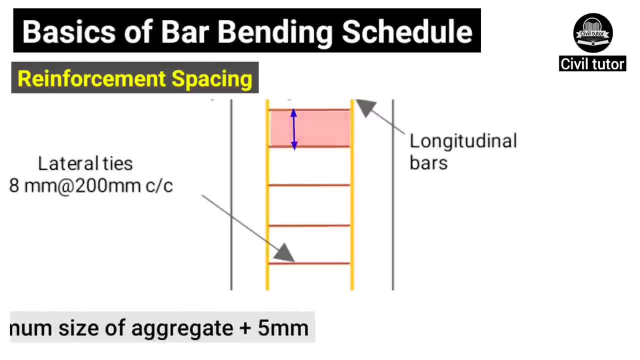 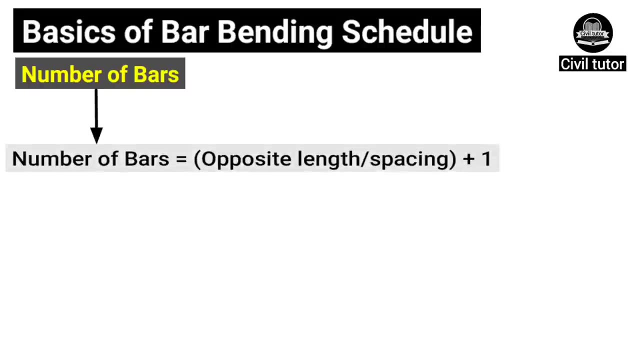 the steel bars with concrete, The minimum spacing between two bars should be at least equal to maximum size of aggregate, with a margin of 5 mm. The next topic is about number of bars. Number of bars are calculated by using the formula Opposite length upon spacing plus 1.. 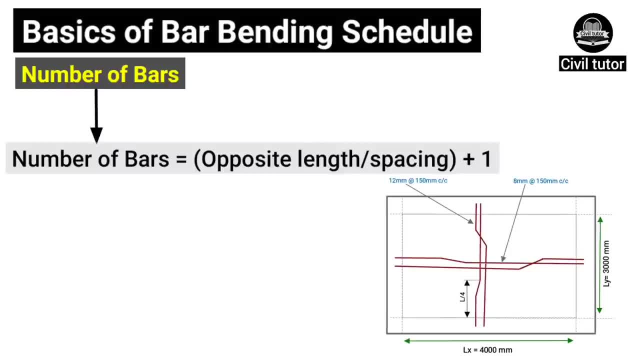 For example, if we have a slab of dimensions Lx into Ly, number of bars along Lx will be equal to Ly upon spacing plus 1.. Similarly, the number of bars along Ly will be equal to Lx upon spacing plus 1..